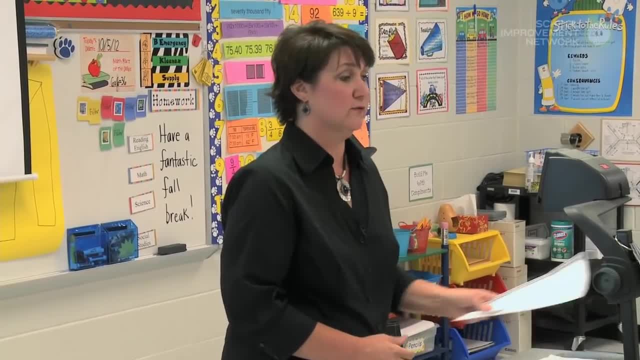 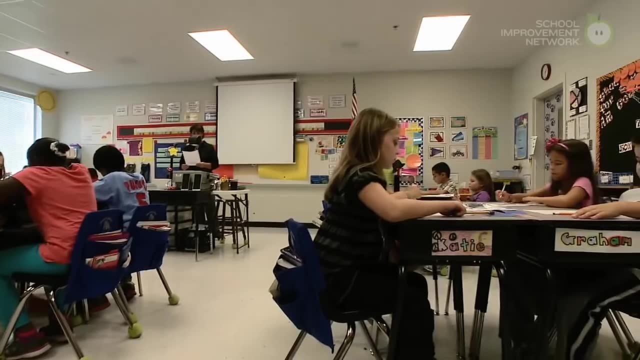 that you found in the text. I will now read it to you. Feel free to also mark something. if you don't feel you got it on your read, Feel free to mark it. at this time, Water striders. Imagine yourself zooming across the top of a pond or lake without sinking in. While this might be, 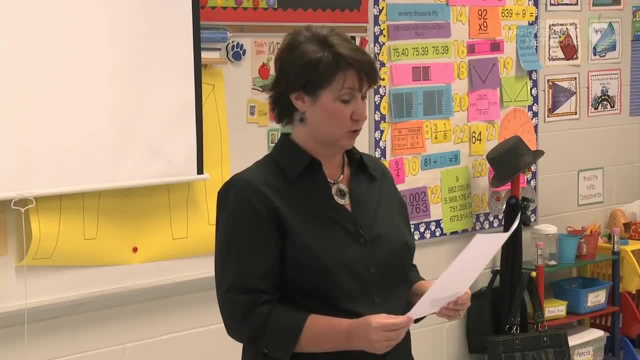 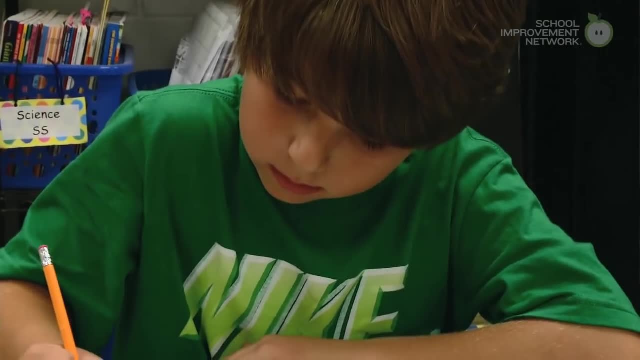 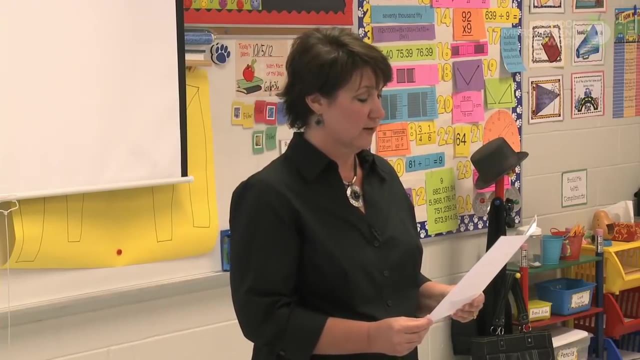 hard for you to do, it is easy for a water strider. A water strider is a water bug that looks like a large mosquito. What makes it different from a mosquito, however, is the fact that it can walk across the water. You can find water striders on the surface of some ponds, marshes and still. 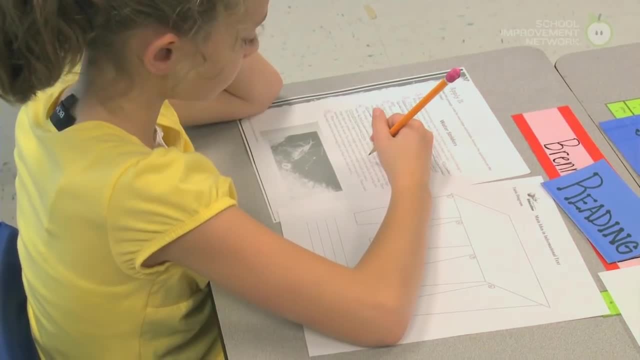 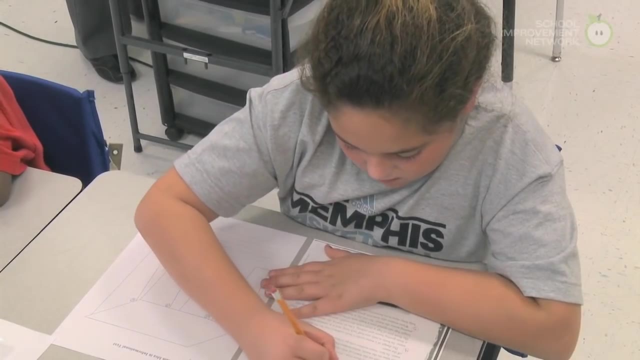 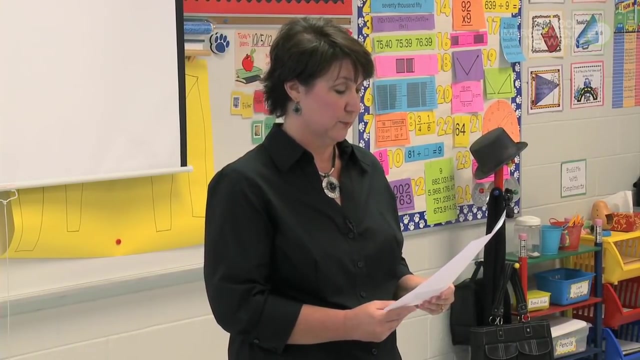 water. Water striders do more than just walk across the water. They also catch and eat their meals on the water as well. Additionally, because they spend more of their time on the water, water striders feed mostly on other insects that live near water. In fact, water striders only go inland when rain. 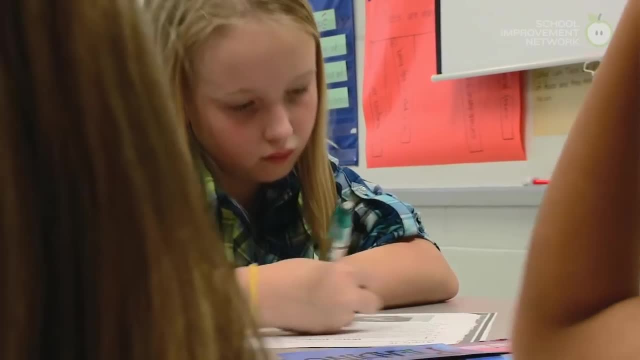 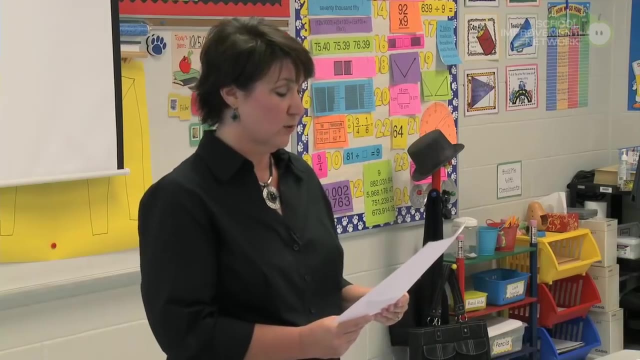 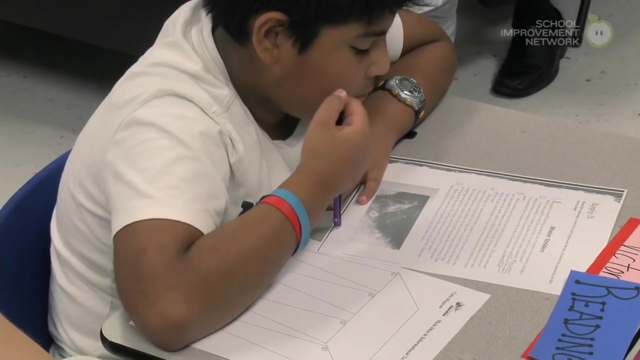 or strong winds force them off the water. The design of a water strider's body makes it easy for the insect to walk on the water. Its body is only one half inch long and it is covered with scales that keep it from getting heavy and sinking. Like all insects, the water strider has six legs. The front pair of legs is 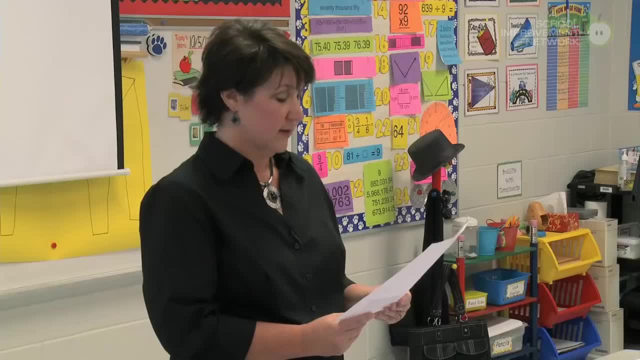 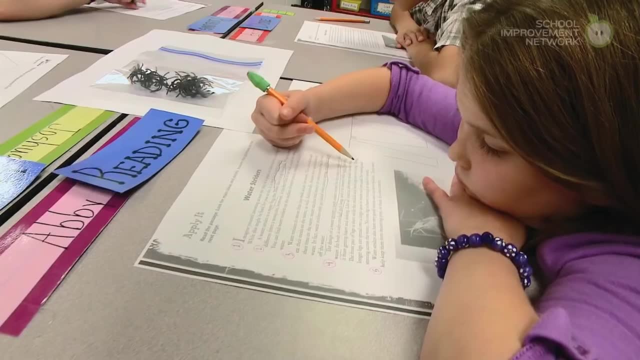 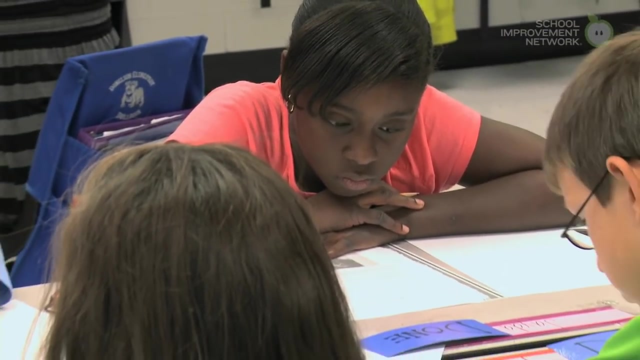 short, while the middle and back legs are very long. The longer legs can spread over a larger area of water and are useful for rowing and steering across the water. No one leg is heavy enough to sink the insect. The water strider has a very good vision and can move quickly. These traits help keep them from. 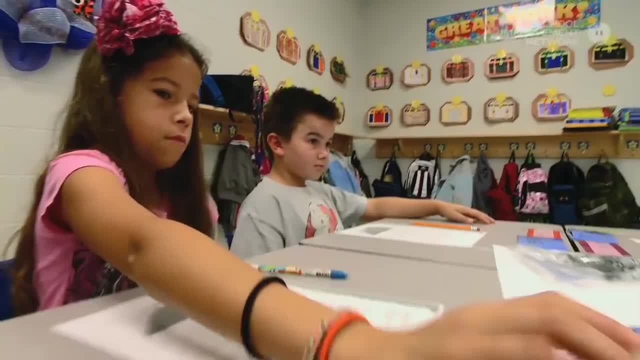 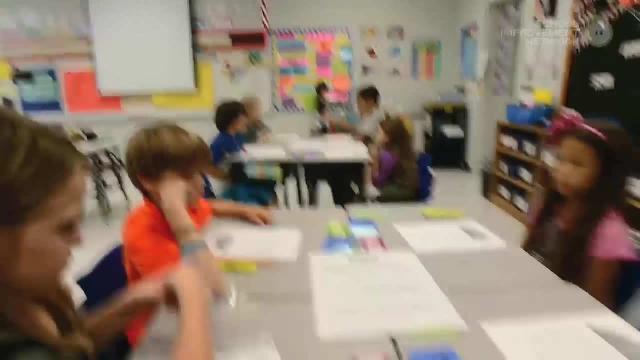 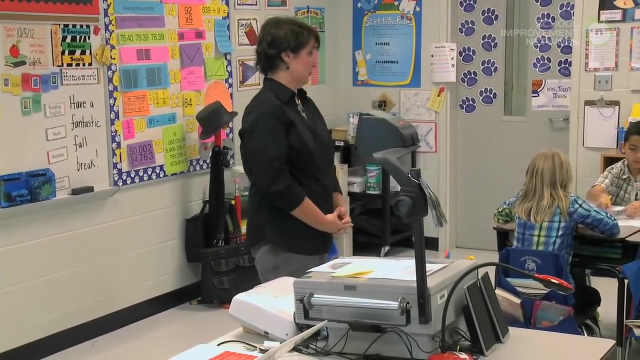 becoming prey or food for other insects. Okay, now it's time for us to work on some text-dependent questions. We are going to play bingo. while we answer the questions today, You have some spiders that you're going to use as your markers. 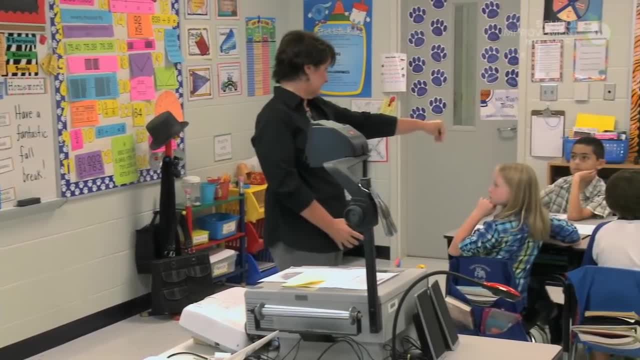 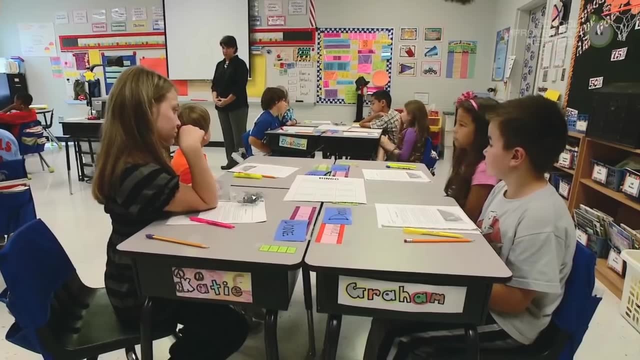 Here's how the game will be played. Your entire group is one team. I will tell you what row or column we're working on at that time. Whenever I show you what row or column we're working on, your team is going to try to find the answers. 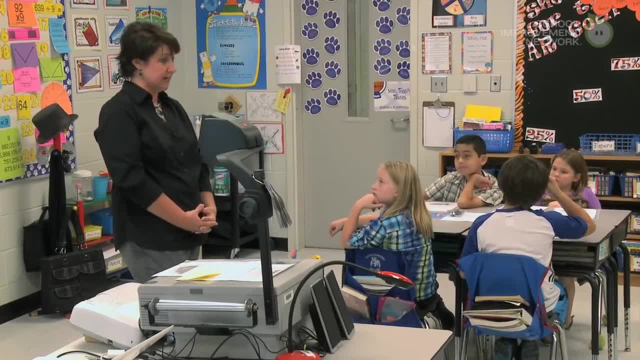 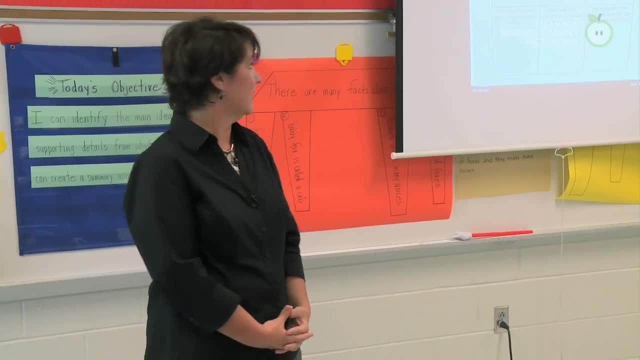 to those questions. They must be highlighted in the text and you must be able to tell me where you found it, with the paragraph and the sentence number. Here we go. The first thing we're going to work on is, across the top, What insects does a wa? 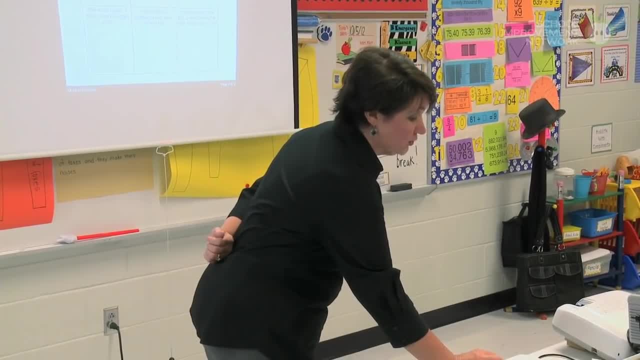 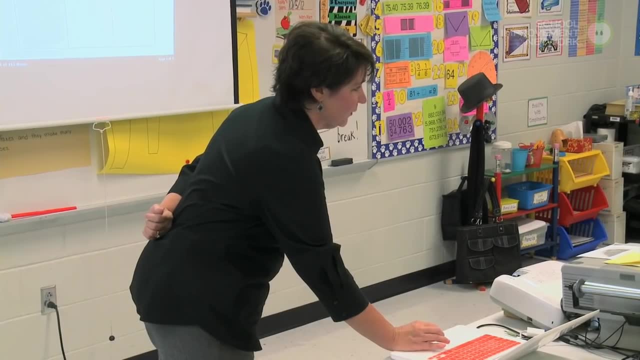 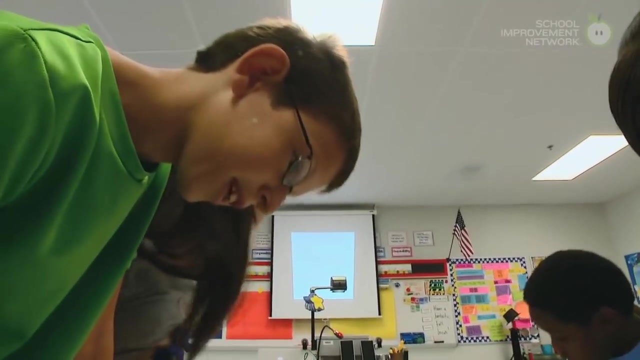 What insect does a water strider resemble? How would you describe the size of a water strider? What fact can you select to show the speed of a water strider? Go, A water spider, A large mosquito. It looks like a large mosquito. 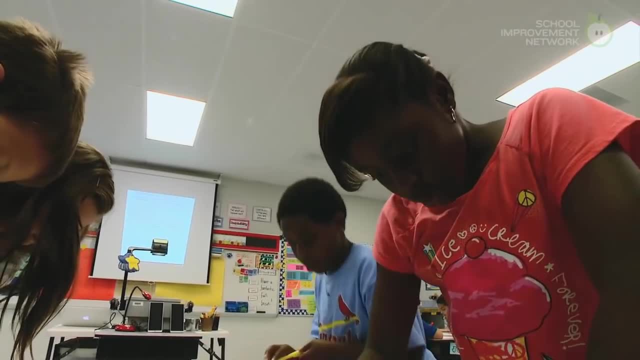 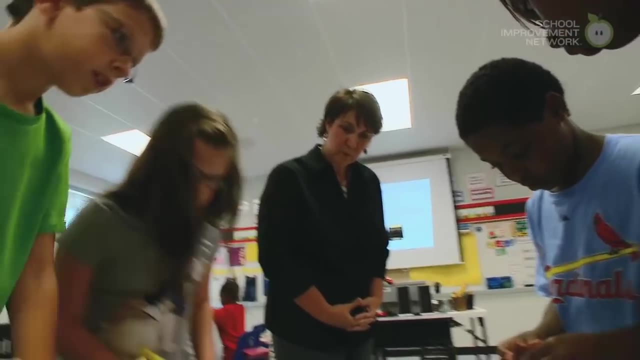 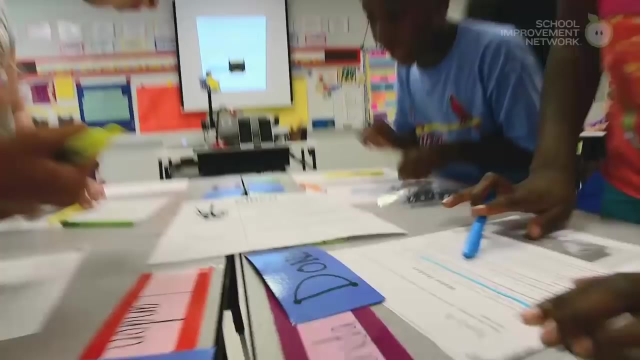 A water strider. Yeah, Yeah, Okay, so put a spider right there. What's your answer going to be? Which answer? Oh, A large mosquito. A large mosquito. Okay, How would you describe the size of a water strider? 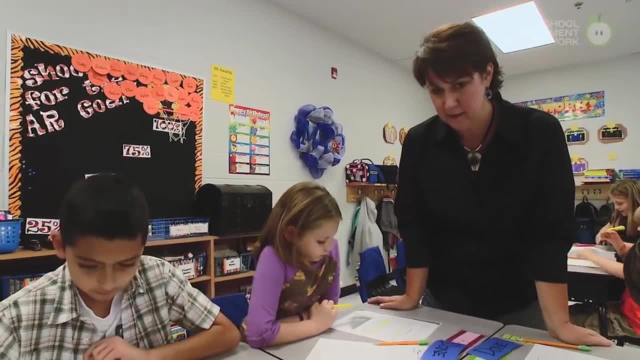 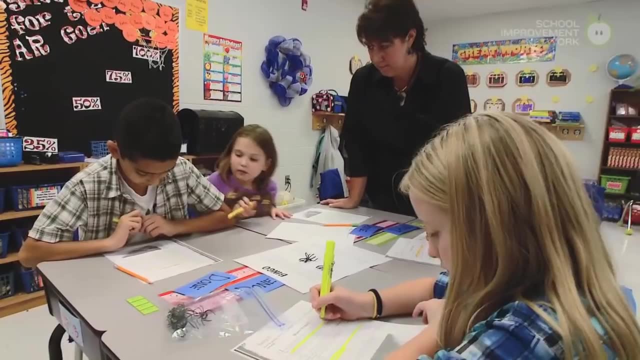 You're going to find it in the text. You have to be able to highlight it to use it for an answer. What fact can you select to show the speed of a water strider? Water strider. Abby has an answer. Share it, Abby. What did you see? 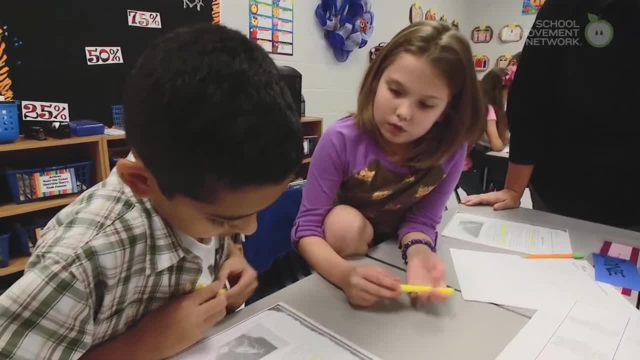 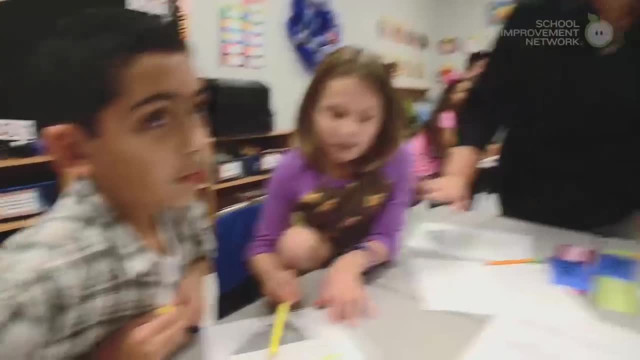 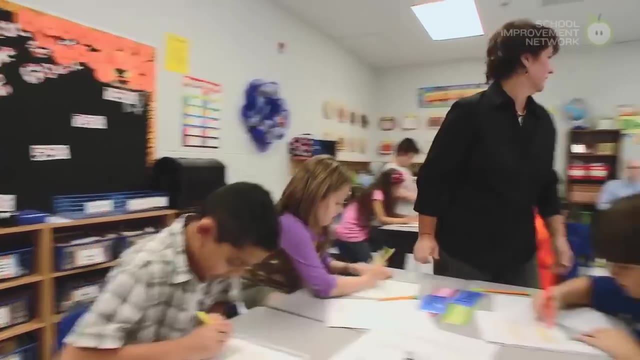 I saw sentence five, group one. I think it's in paragraph three: Water striders also have Striders, Go on and finish Good vision and can move quickly. Awesome job, Awesome. Okay, I heard my first group, Water striders. I heard it. 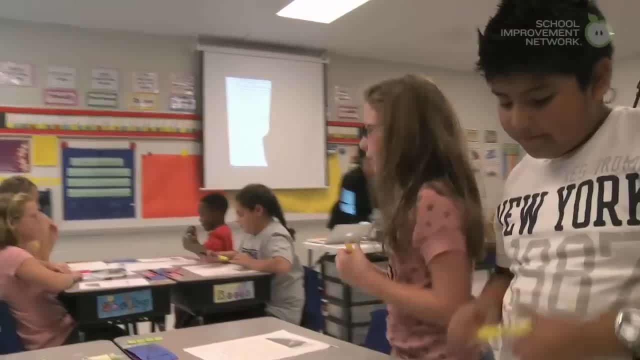 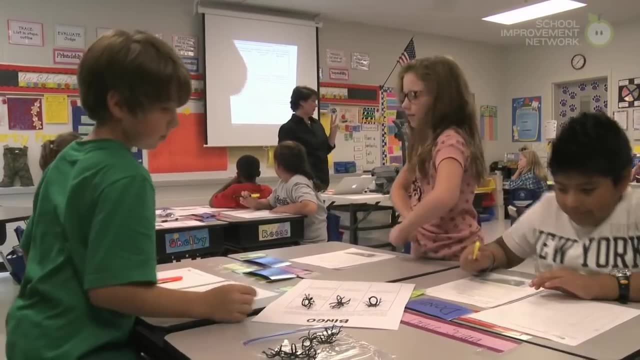 Okay, let's see if they've got it. Now they're going to help you out because, remember, when we respond, the first thing we do is tell the paragraph, then the sentence number, then we give our fact, but then we answer our question And I'm going to type the answer up here. 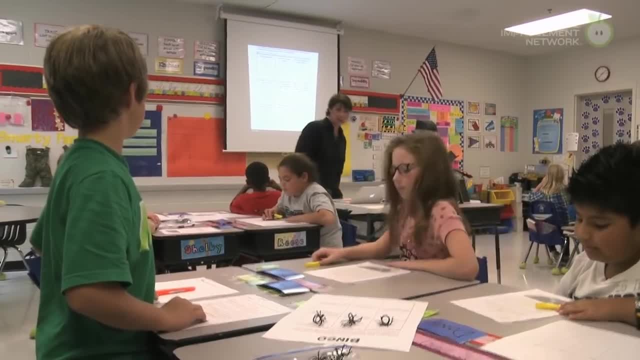 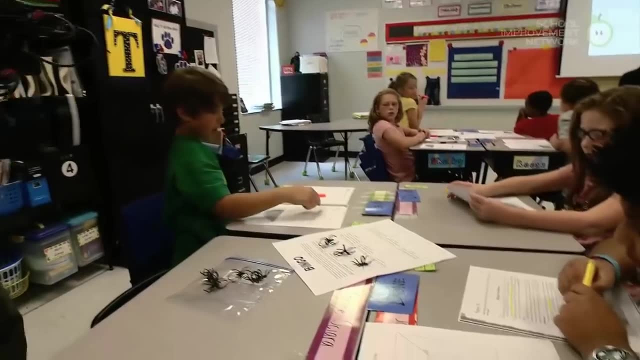 That way you'll make sure you've highlighted the correct section. Here we go. Which insect does a water strider resemble, Hudson? can you tell me where you found that answer? Paragraph two, sentence one: A water strider is a water bug that looks like a large mosquito. 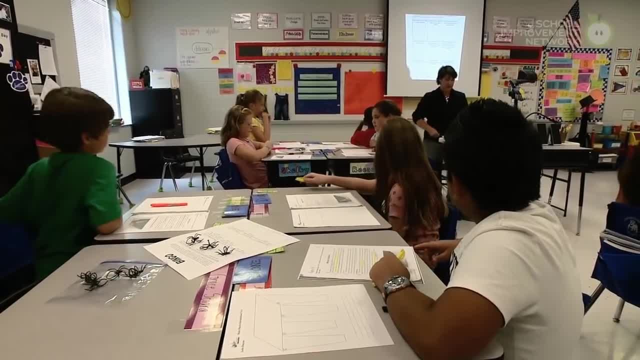 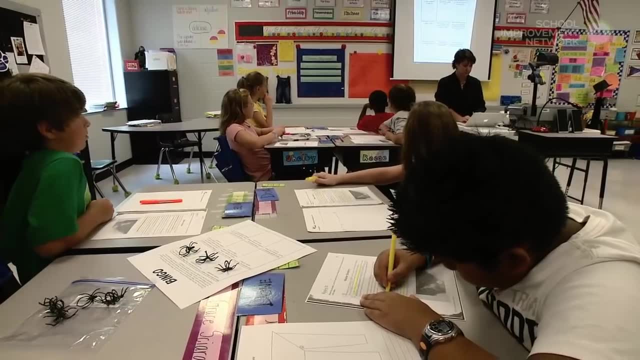 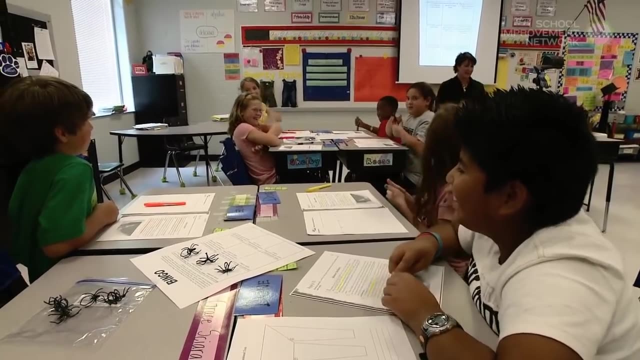 Okay, so he said paragraph two, sentence one, And what is your answer then? A large mosquito, A large mosquito, A large mosquito, He is correct, Looking good. Next one: How would you describe the size of a water strider? 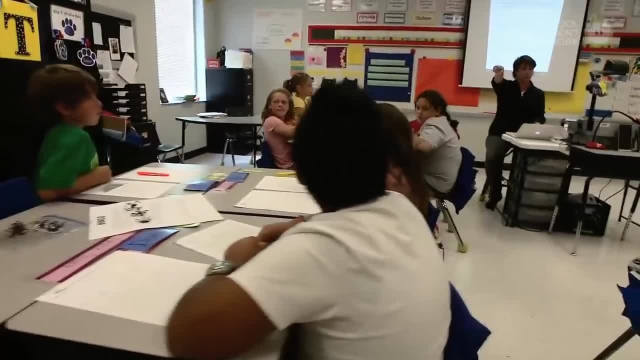 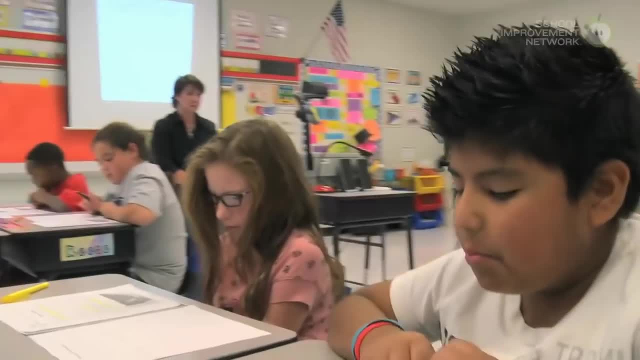 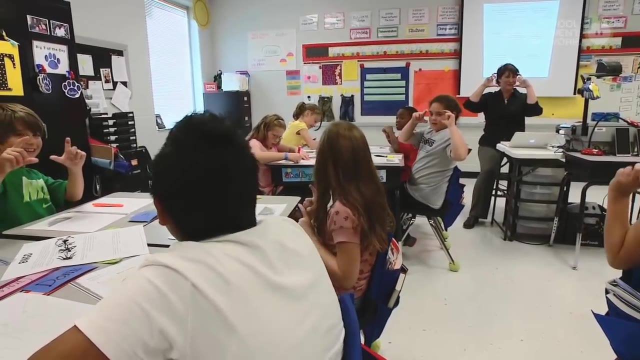 How would you describe the size? I'm still on this table because they were the first group. Victor, can you answer that question for us? Paragraph four, the second sentence, says: its body is only one-half inch long, Ready, Looking good. 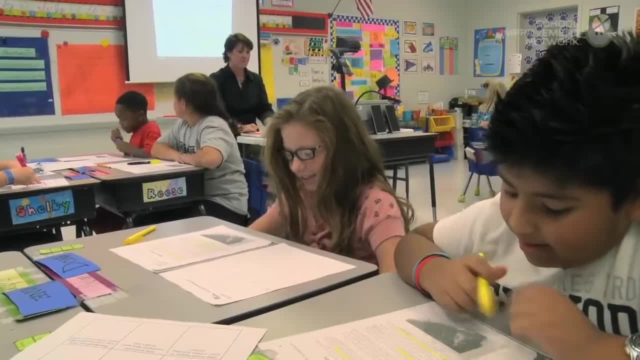 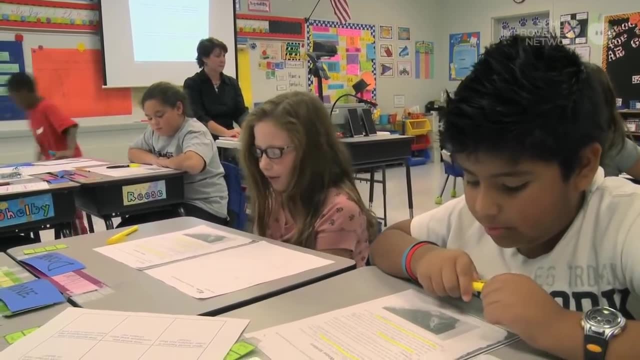 Two out of three. Let's see if they can get the last one. What fact can you select to show the speed of a water strider? Dylan, it's your turn. Paragraph five, sentence one, says: water striders also have very good vision and can move quickly. 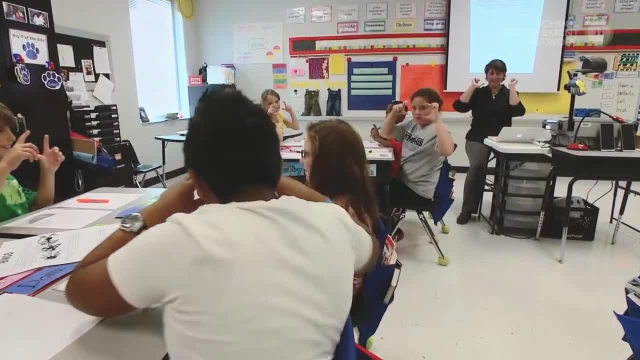 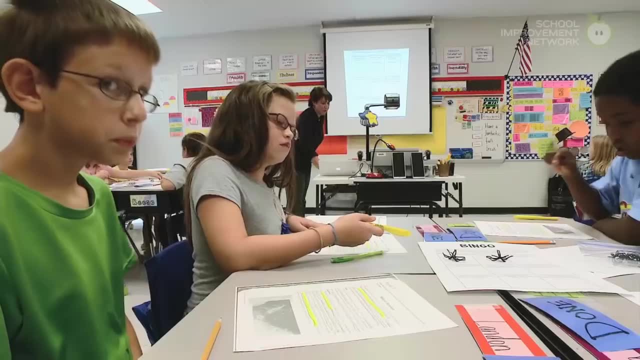 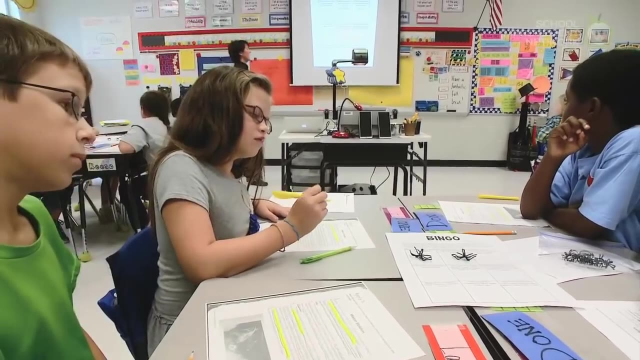 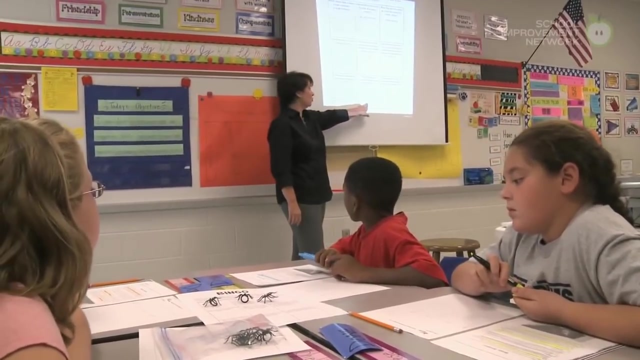 She got it Ready, Looking good, Great job. Now we are moving to the center column. The next question is: Since the title of the article is Water Striders, would you find a water strider on land? Next one: How would you summarize what water striders eat? 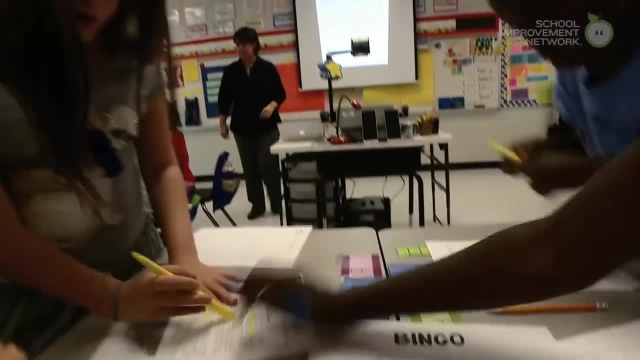 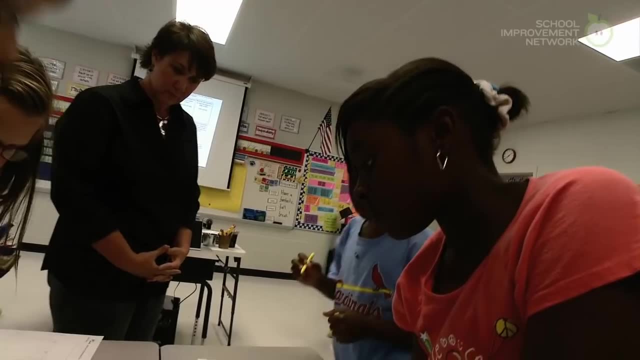 Go. It says that most of its time it says We still have to do this one. No, we don't. No, She only said this column right now, But you'll need to highlight that answer to be able to put a spider in there. 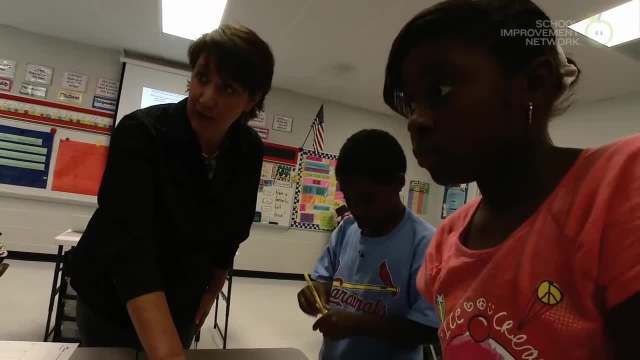 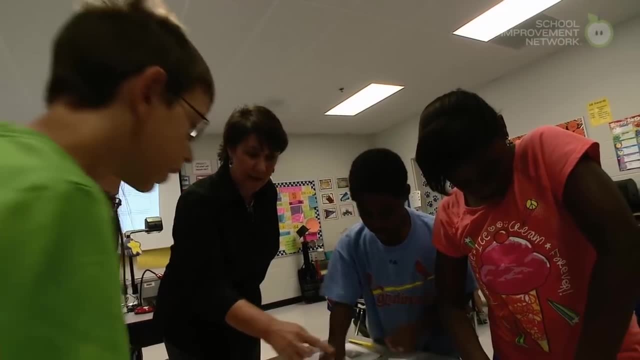 You'd have to highlight that. Did you highlight it when we went over it? Us three did. Okay, make sure your whole group has that highlighted and you can put you a spider there. If not, in a minute you won't be able to use it. 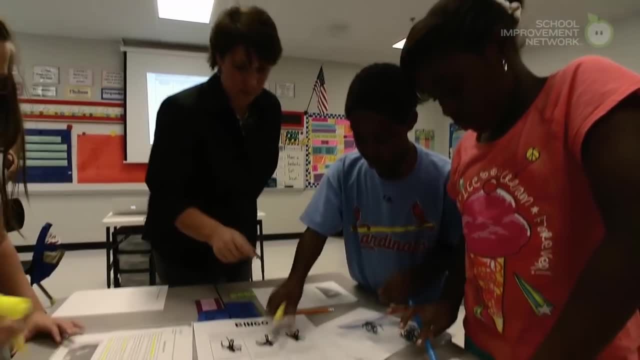 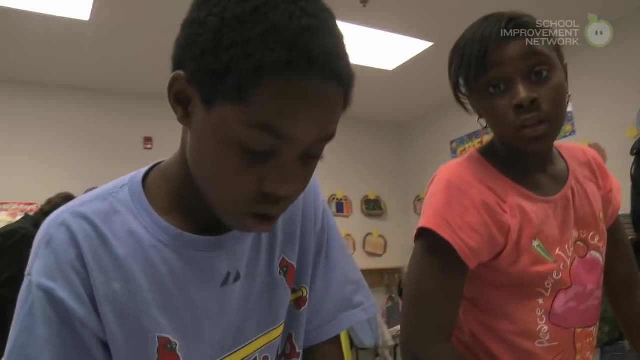 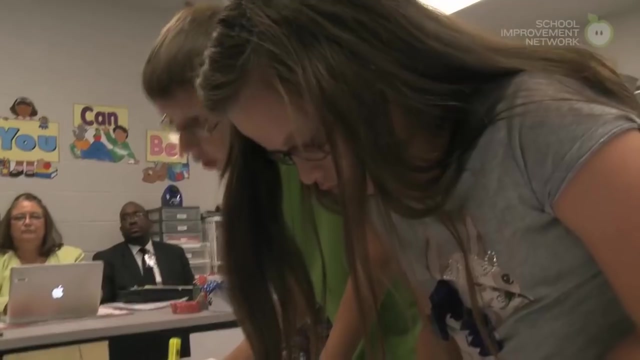 Does everyone have it Okay? Okay, now, you can Now go. It says they go inland when rain and strong winds wash them off the water. No, it says they spend more of their time on water. Yeah, And we think that you possibly could find it. 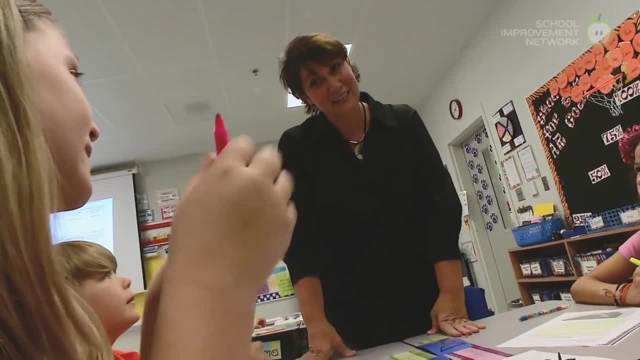 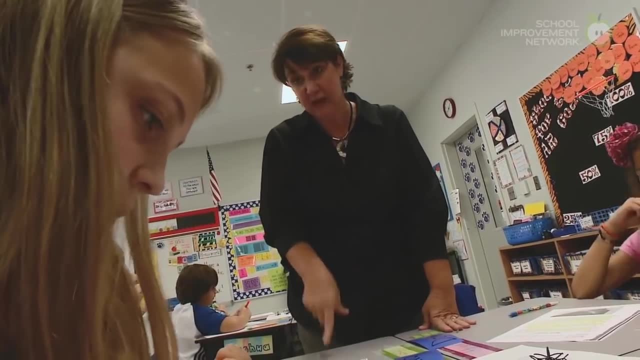 Impossibly Okay. but remember we worked on opinions and our prior knowledge. We can't bring any of that to the text, So you have to be able to find it in that passage to highlight it. It says it spends most of their time. 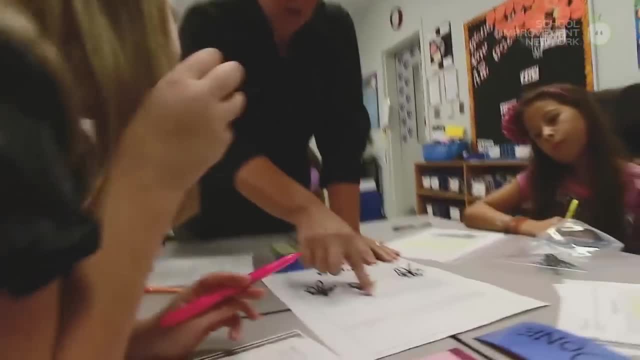 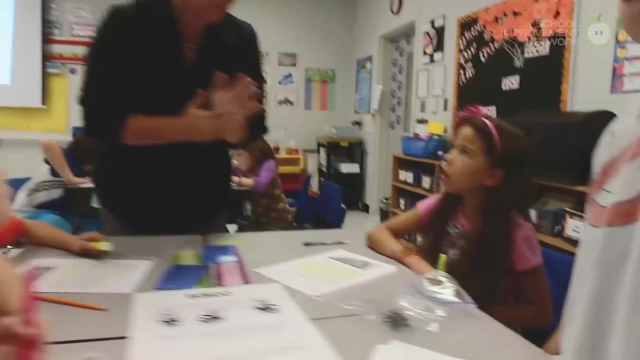 Okay, but the question is: look, since the title of the article is water striders, would you find a water strider on land? No, Okay, so you're talking about when something pushes it off. Okay, find that, You're getting there. 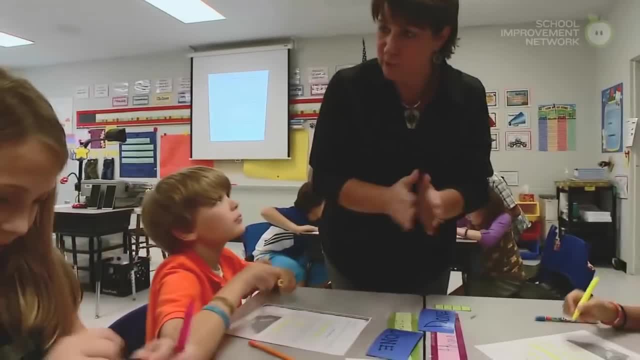 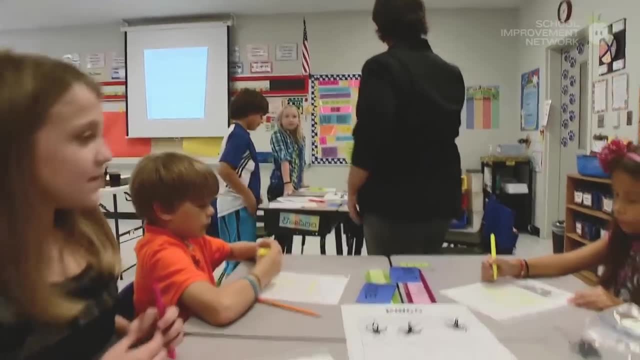 Find it. She said I remember. but now help her Find it. She remembers it. talked about it pushing it off. Oh, I heard one right here. Let's give everyone another second or two to work on it a little bit further, but you are the group that I heard. 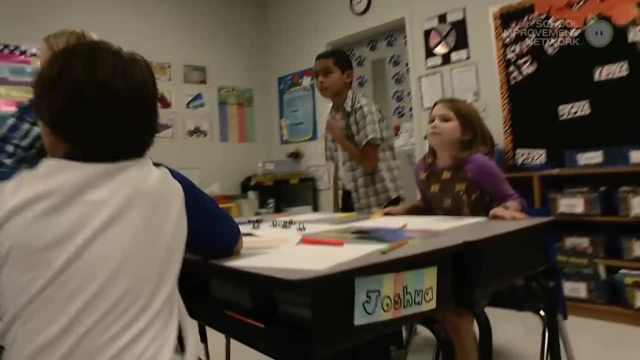 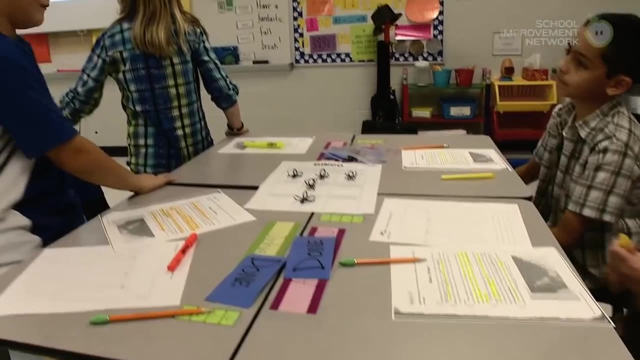 Okay, Okay, stop. Emily's group up here thinks they have the answers. Now remember: if your group didn't get to it, you need to find it. If your group didn't get to it, you need to listen to where you can find the information in the text and highlight it. 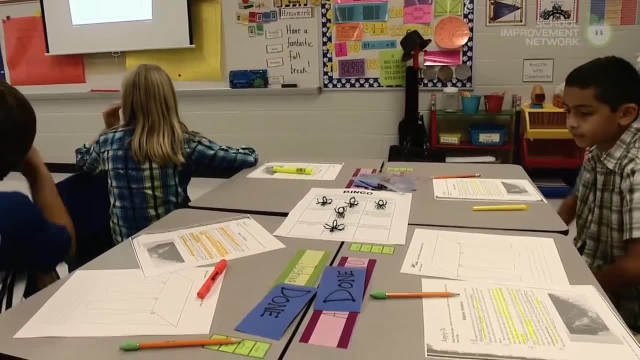 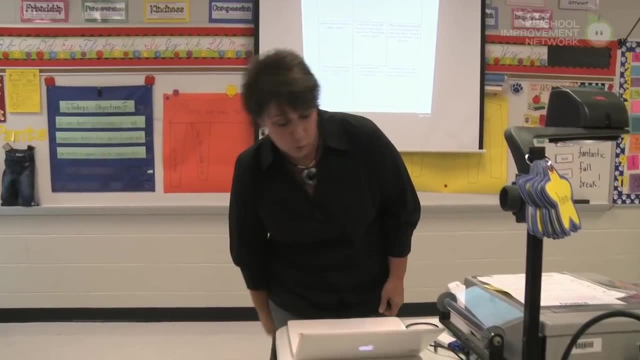 If you highlight it, you can give yourself a spider, because you need all the spiders you can get on there. Okay, Emily, here we go. It says, since the title of the article is water striders, would you find a water strider on land? 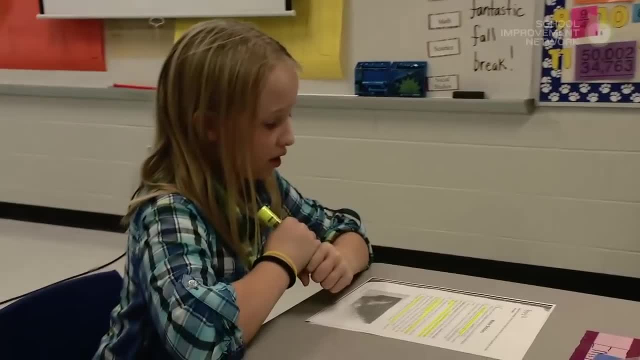 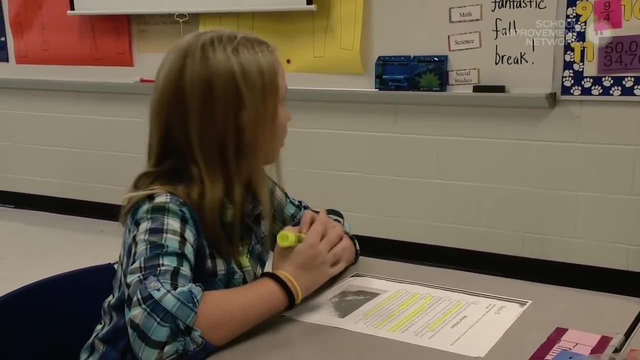 No, because it says in paragraph three, on the last sentence. In fact, water striders only go inland When rain or strong winds force them off the water. That is the text she needed. Now, Emily, let me ask you that question. 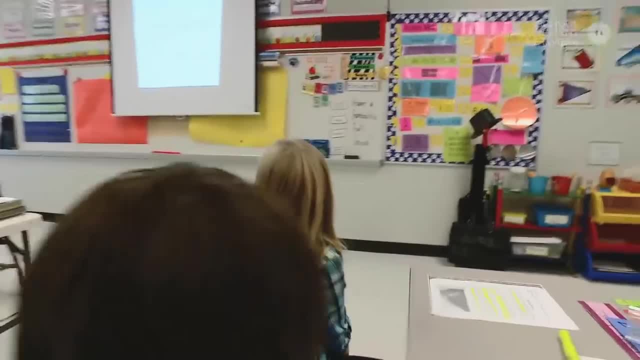 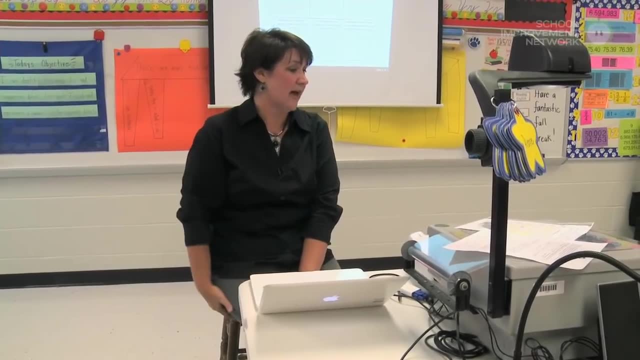 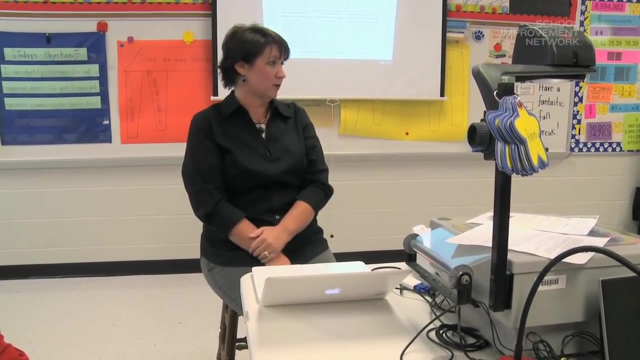 The question is: would you find a water strider on land? No, not usually. Okay, but listen to it one more time. In fact, water striders only go inland when rain or strong wind forces them off the water. Do you know what inland is, Emily? 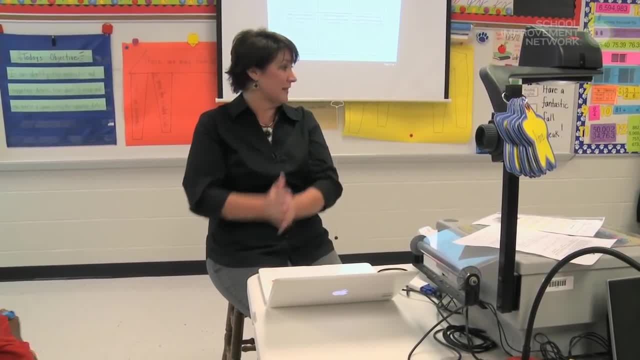 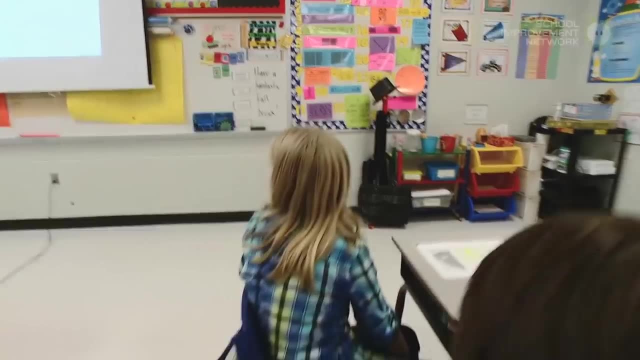 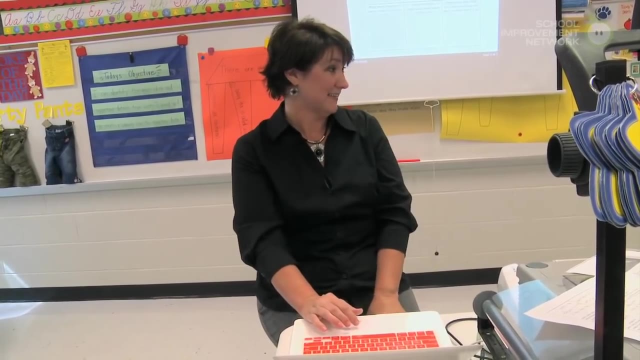 Yes, ma'am, Okay. So will they ever go on land? Yes, when it's raining or it's blowing really hard wind. Okay, when they're forced that way. Even though they're called water striders, you could possibly find them on land. 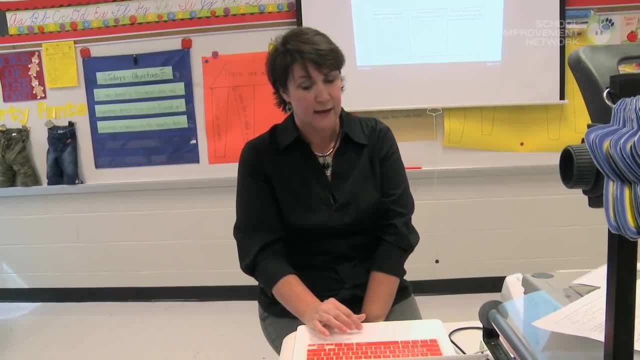 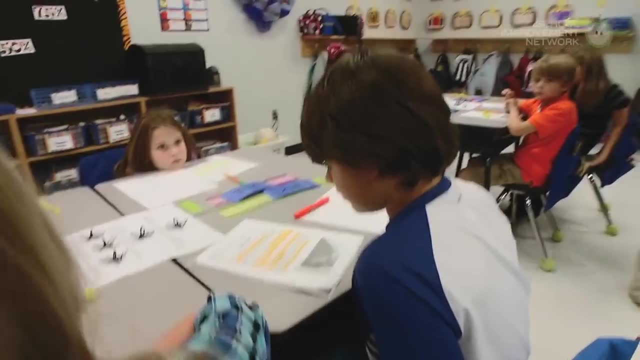 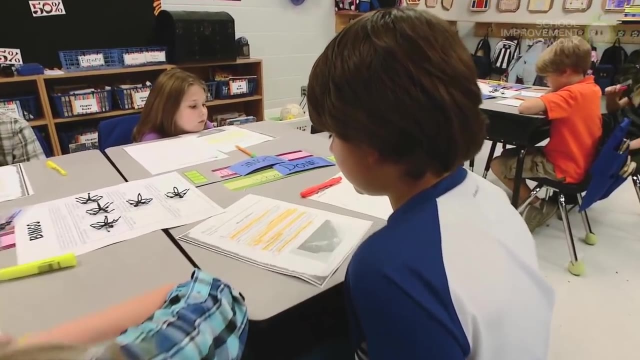 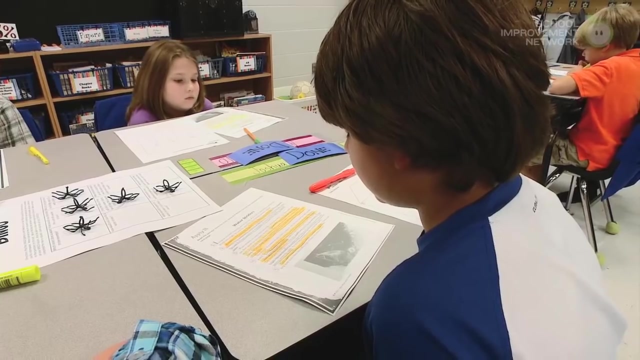 Okay, and next one, Josh, answer this one for me. How would you summarize what water striders eat? In our third sentence it says: additionally, because they spend most of their time on water, Water striders feed mostly on insects that live near water. 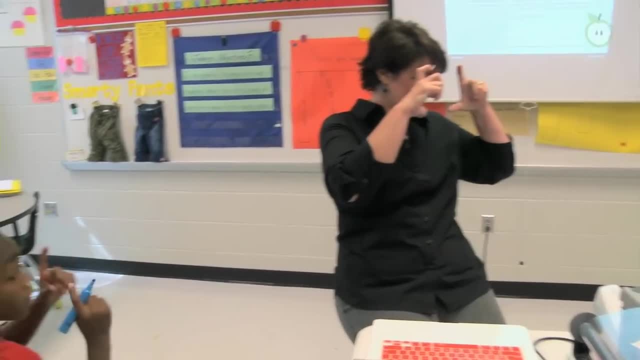 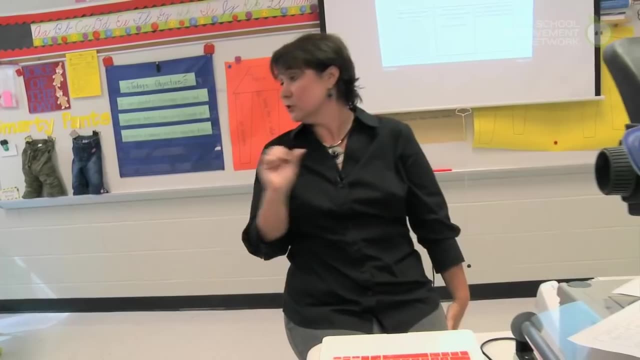 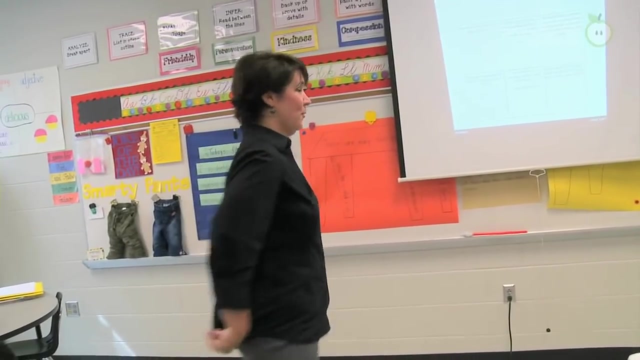 Let's give both Emily and Josh our cheer. Looking good Again. if you highlighted that, even if your group didn't make it, you can put you a spider there. Next row, Here we go, Bottom row, Bottom row. What would happen if water striders lost their vision? 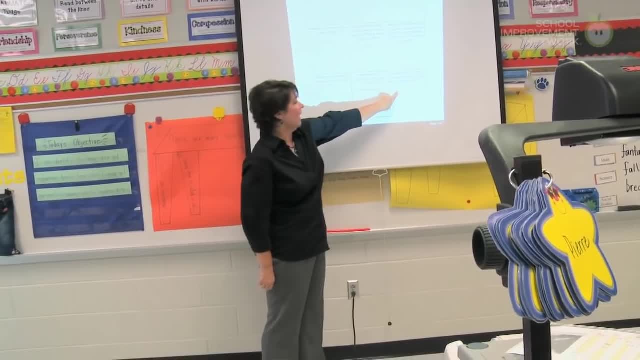 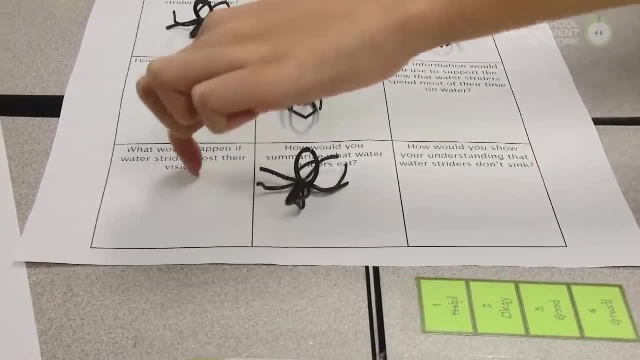 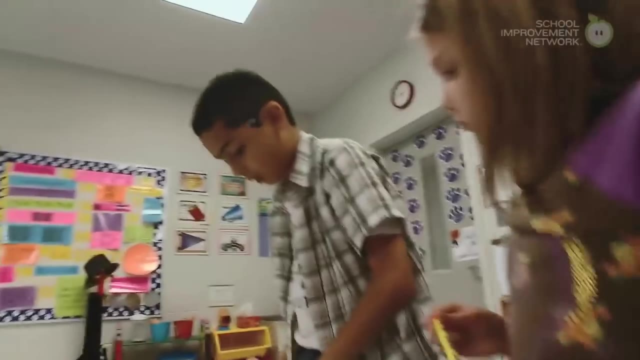 You should already have this one answered. And how would you show your understanding that water striders don't sink? Go On this one. water striders also have very good vision and can move. Yeah, but that doesn't say what would happen. 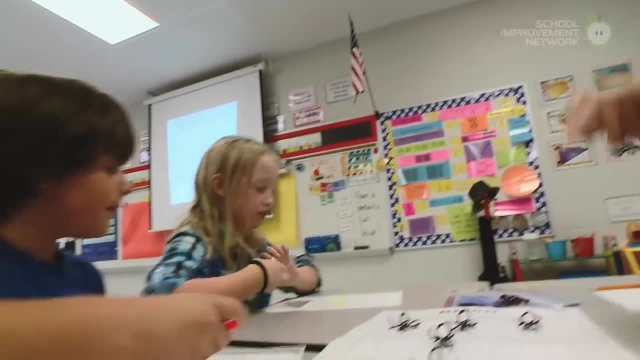 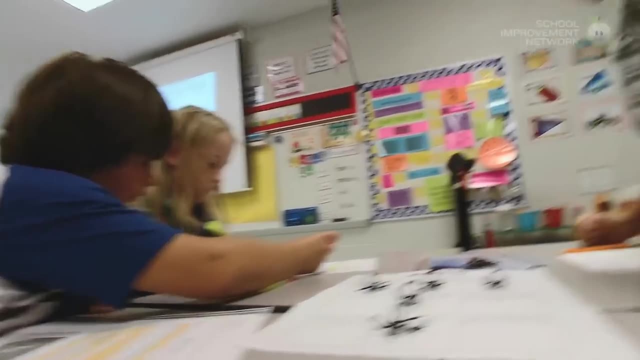 Yeah, if water striders would walk On the day I asked you to trade to the park, we'd become food for the park. Josh, that's wrong. It's wrong. Josh, Josh, that is wrong. I have to say that's wrong. 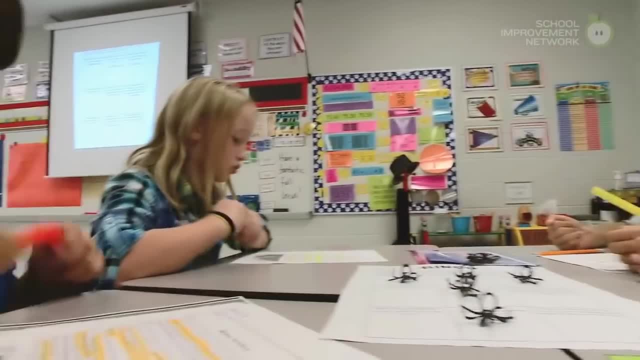 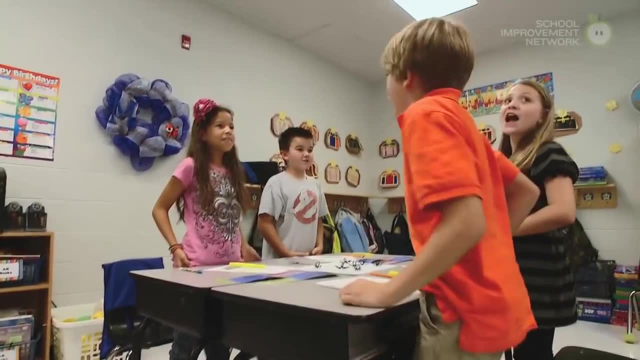 It doesn't help because it says: these traits keep them from becoming food for the park. Our striders lost their vision. All right, stop, We've got three more. We've got another group. I like how we have different groups finishing. 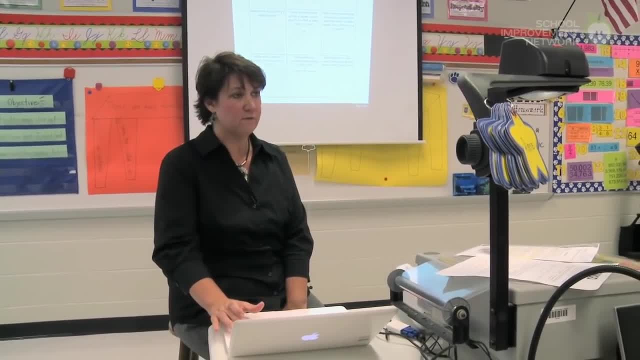 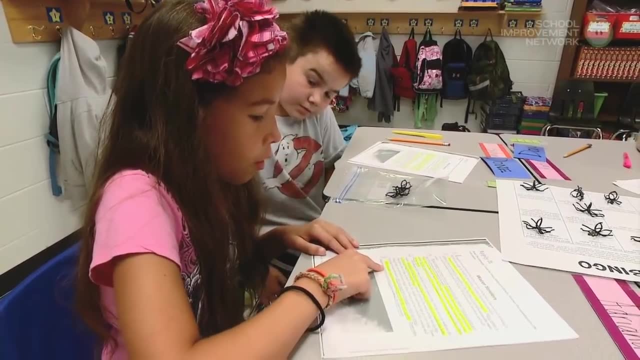 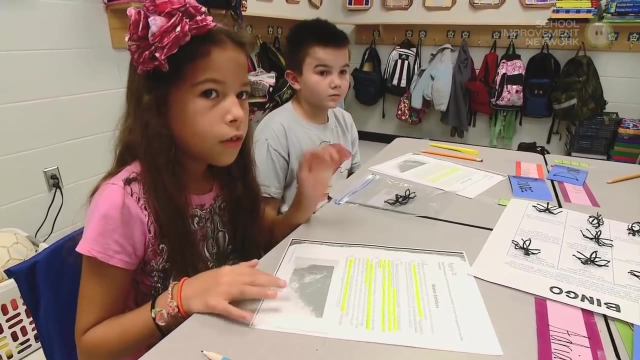 What would happen if water striders lost their vision? Adriana, share with us where you found that answer. In paragraph five, sentence one, it says: water striders also have very good vision and can move quickly. Okay, so what would be your answer to the question? what would happen if water striders lost their vision? 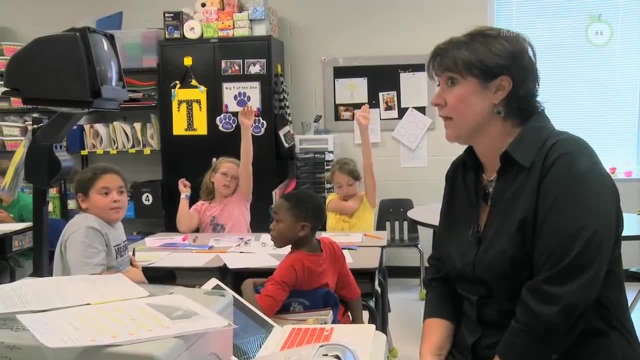 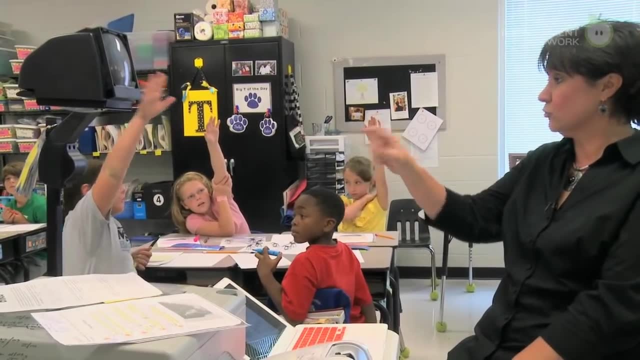 They wouldn't be able to move very quickly. We're thinking a little deeper, though. They lost their vision. This is going to have a bigger impact on their lives. Okay, let's let Ella's group help us out on that. They highlighted a different fact, and see if this will change your view here. 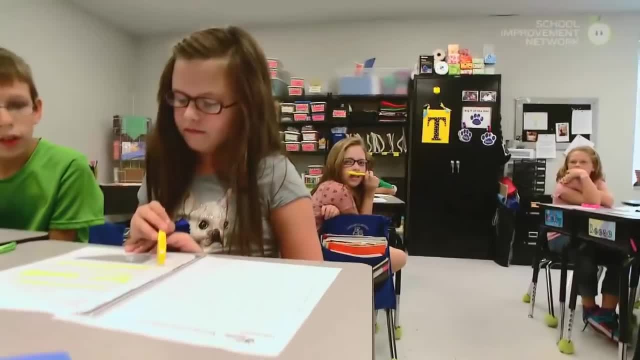 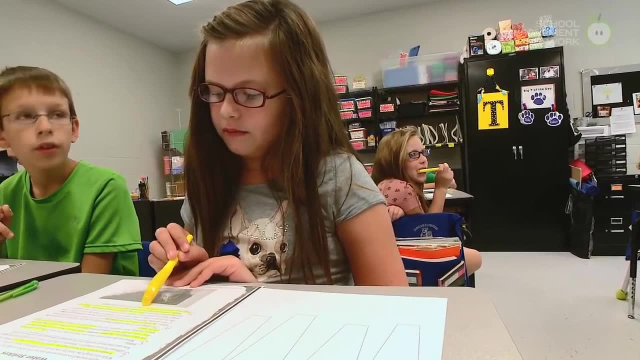 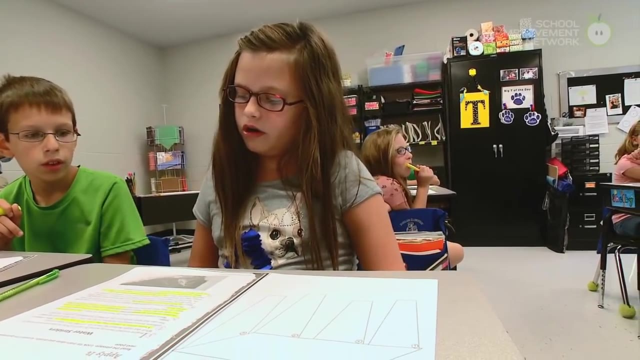 Well, on the paragraph five, the last sentence, it says: these traits help keep from them becoming prey. and if they lost their vision they'd probably become prey because they wouldn't know where they were and they might come into where the prey is. 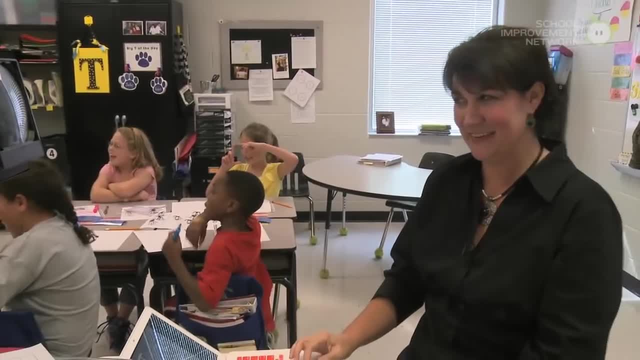 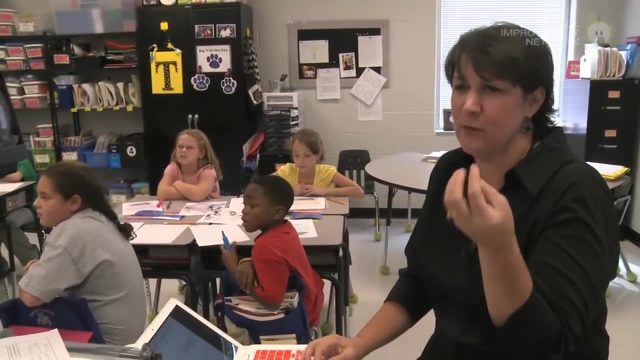 Very good, Let's go ahead and give her the cheer. Looking good. Does that group see how that answer got changed? You were right. They're not going to be able to move as fast. Okay, but is that the most important fact? 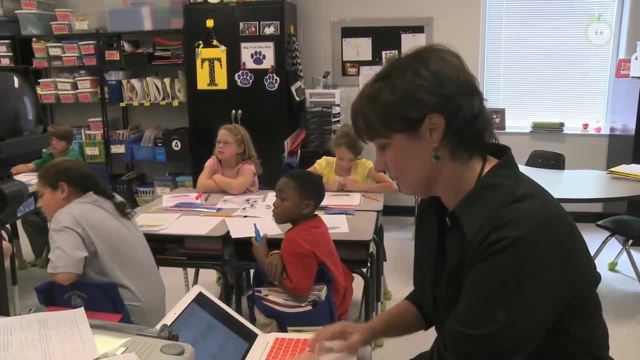 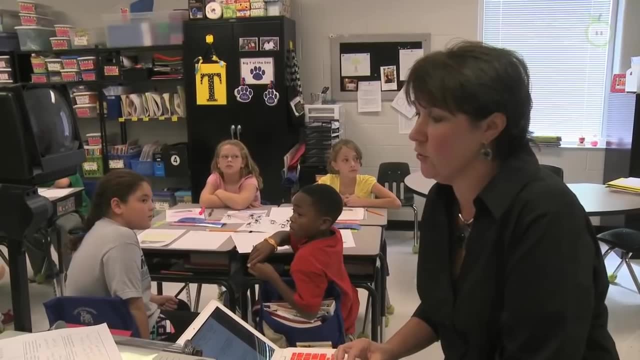 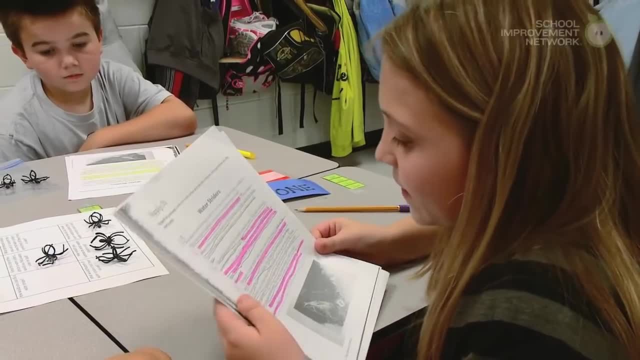 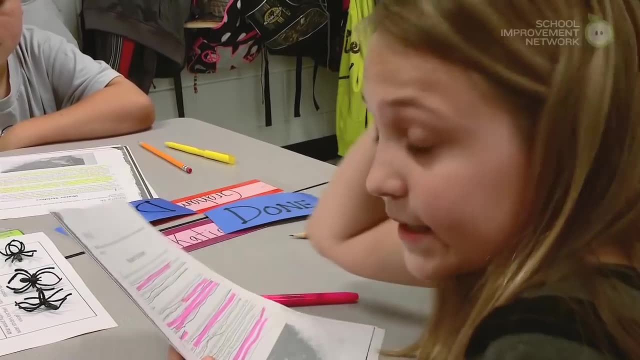 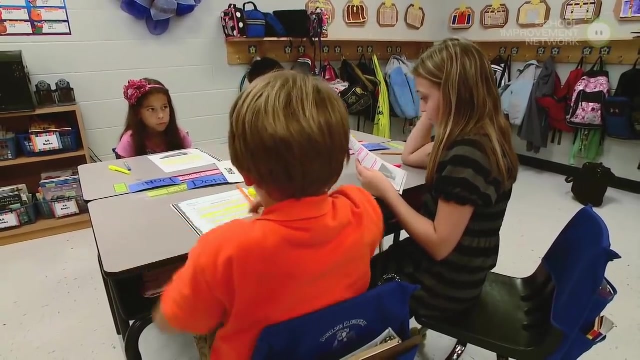 Where did y'all find your information? Their body is only one-half inch long and it's covered with scales that would keep them from heavy sinking. Okay, so that's paragraph four. It's sentence two. Okay, I agree. That kind of shows you they're not going to sink. 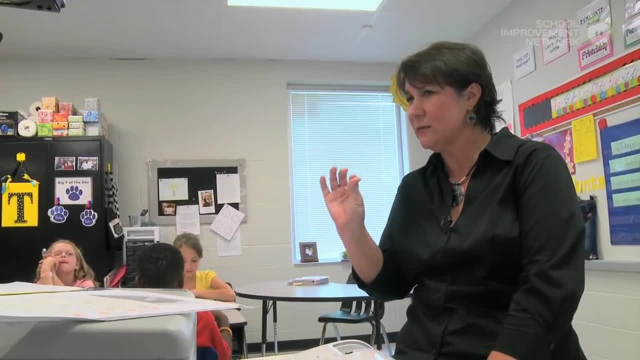 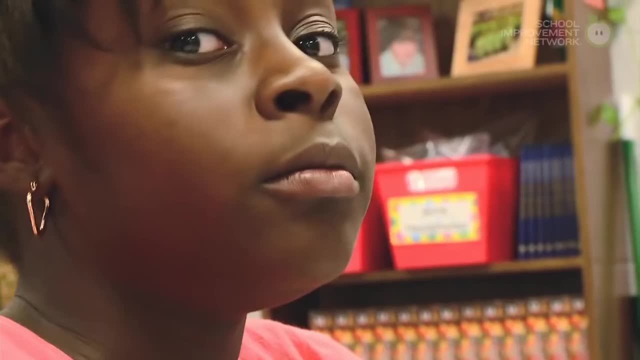 I feel like another group got another fact that was just a little bit stronger. You're not wrong. You are not wrong, But let's see if someone can support it a little bit more. Jada, can you share that with us please? 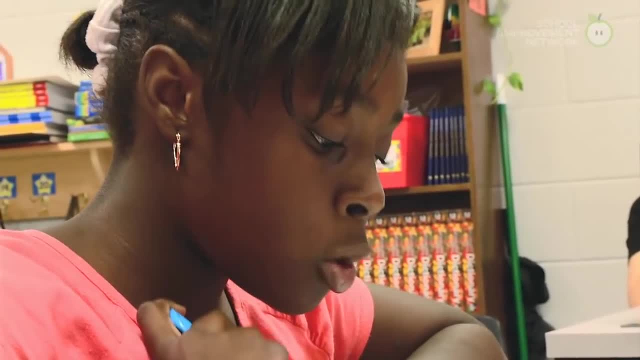 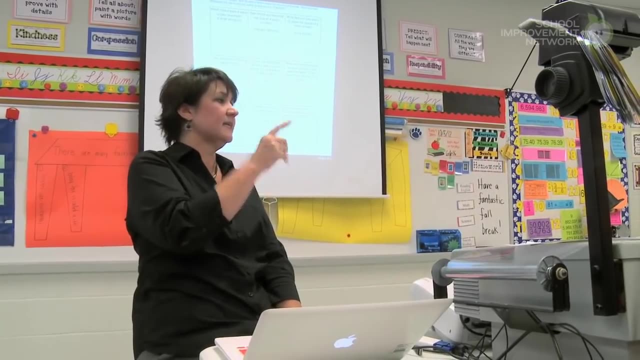 In paragraph four of the last sentence, it says: no one leg is heavy enough to sink the insect. Okay, so we know it's not going to sink because not even one of its legs is heavy enough to sink it. All right, I guess you can tell what we have left. 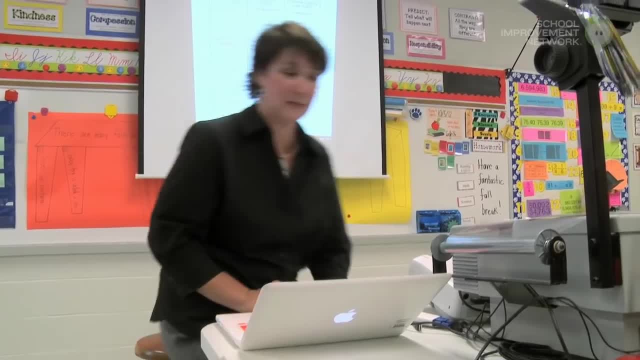 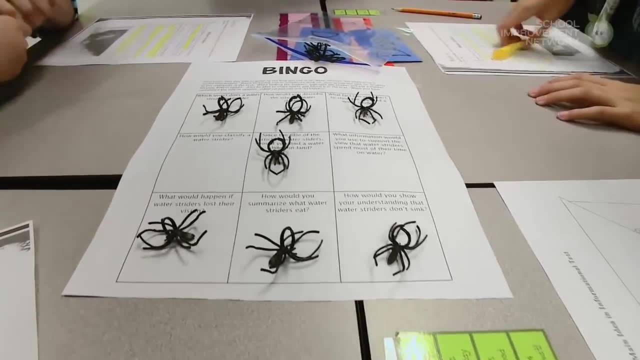 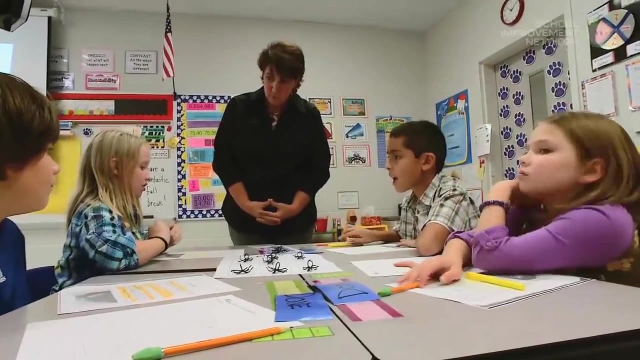 The middle. The middle, Two questions. You may go, Let's see if another group can get it. Okay, can you share with your group what classify means? Classify means like: how would you describe it? Okay, a little more than that. 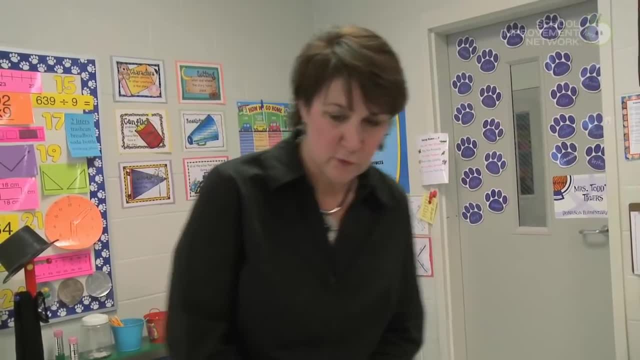 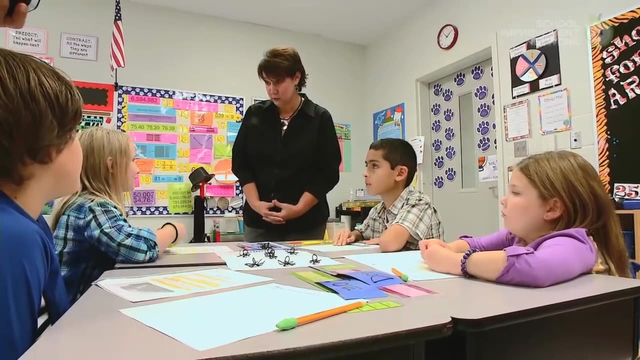 A classification. Okay, think of food. Think of food. Are there different types of food? Okay, name some types of food. for me, A sandwich. Okay, fruit Meat. Do you have anything else? Do you have any sugar? 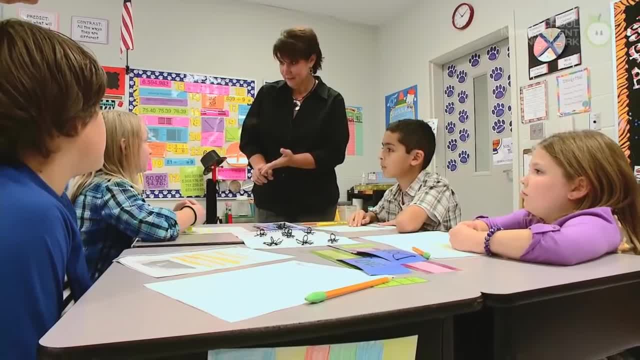 Nothing sweet, Not a brownie or anything- A granola bar. Those are classifications. Now you're looking for a classification, A type. There's something in the text that's going to help you with that. Okay, Okay, Okay. 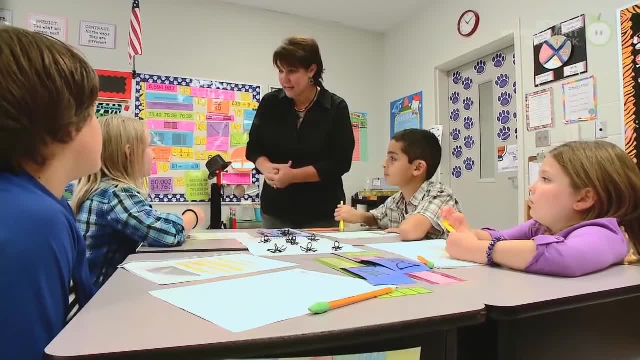 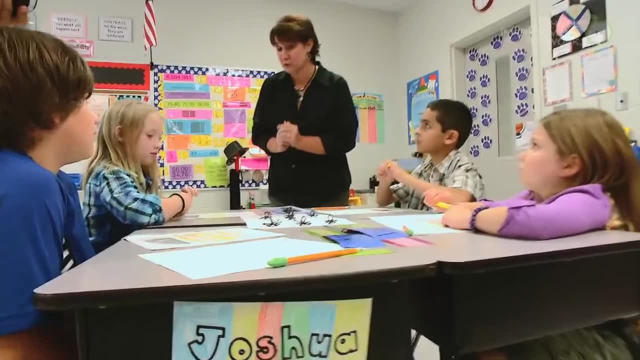 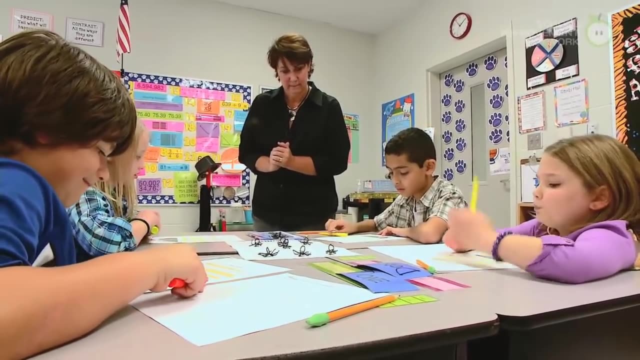 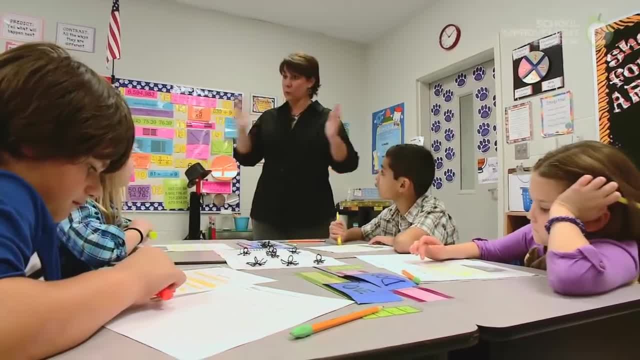 Do you want to see something? Think about like a food, food, something like that. How would you classify it? Think about like the big word food. and then we broke it into like categories. What category is a water strider going to fit into? 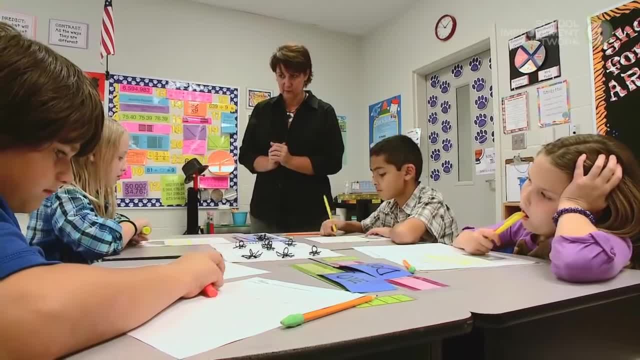 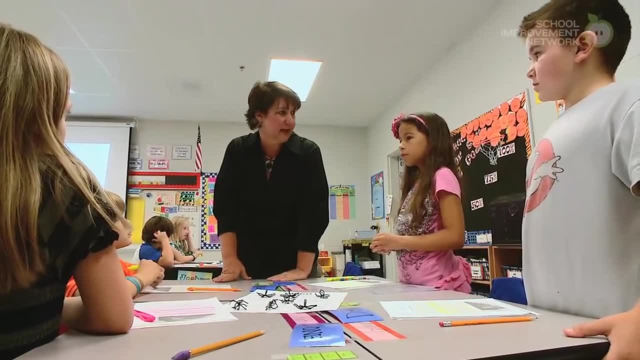 Are we needing to work on classify over here? Okay, so we put it into categories. I want you to take the word classify and think of a category. I wonder what a water strider. what category Pay would it fall into in this text? 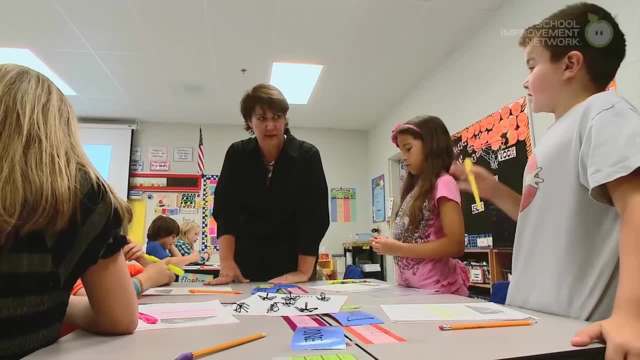 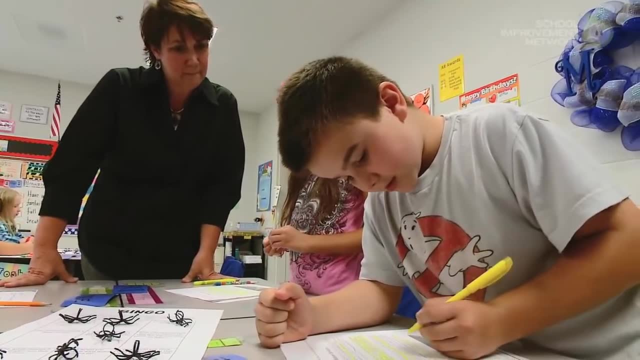 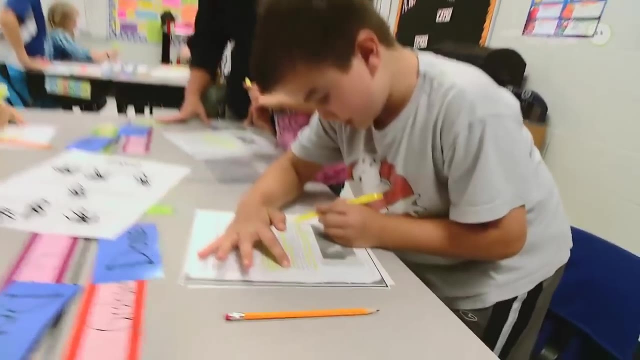 It tells you. It tells you what that is. Where did you find that? Let him find it for you. Where did you find that, Graham? What category are we going to put it in Paragraph, Paragraph four? You're there, bud. 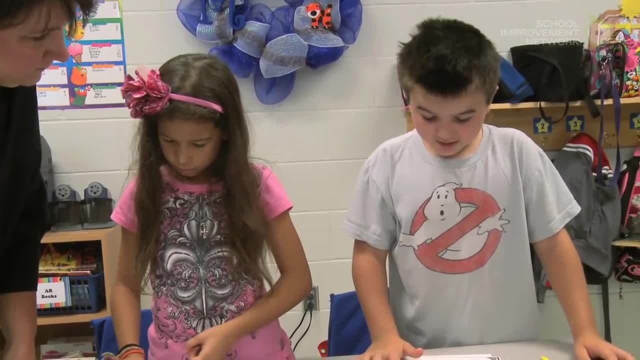 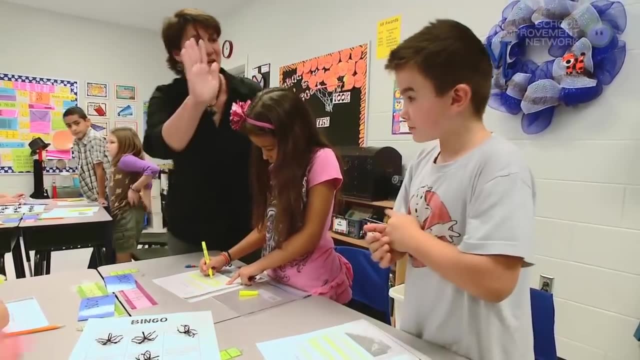 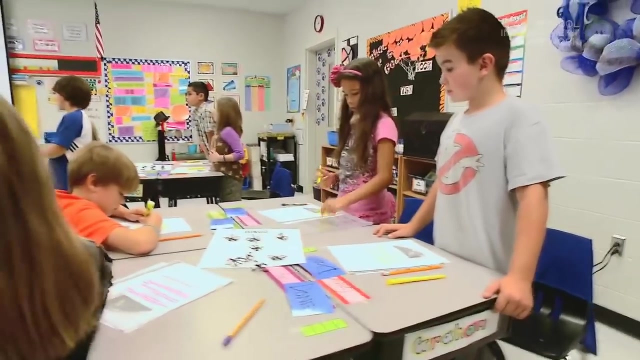 Find it. Like all insects, the water sharder has six legs. Okay, so that was paragraph four, Right here. Like all insects, Graham, give me five. Okay, I had a group over here. I heard them. This one was a little challenging because we had some vocab. 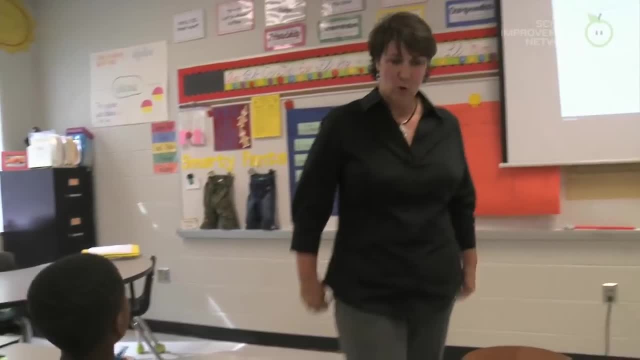 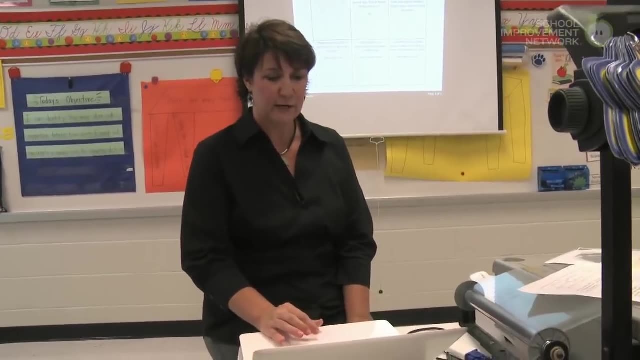 All right, have a seat. Have a seat. I think our board is full. Let's see if we can finish our answers. Classify stumped some people. The word classify, that's some vocab we're going to need to work on. 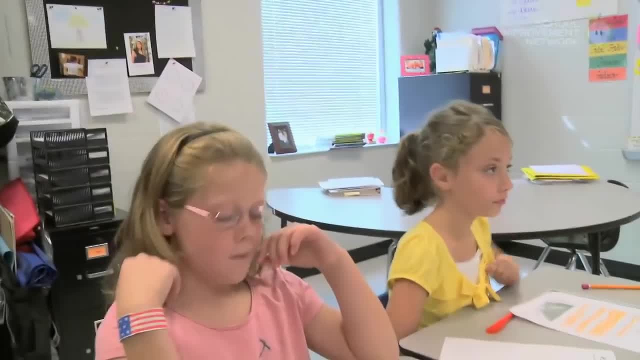 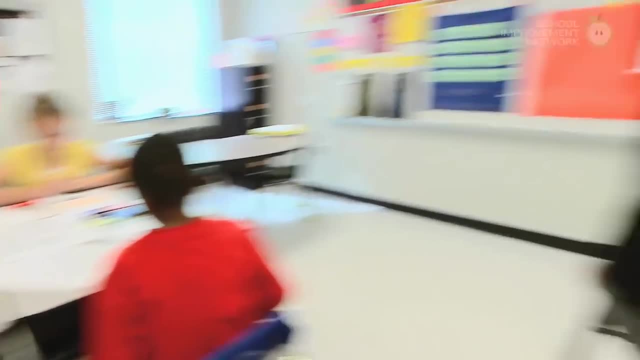 How would you classify a water sharder? Shelby, can you tell me where you found that? We found it in paragraph four, sentence three. Okay, will you read it for me? It says: like all insects, the water sharder has six legs. 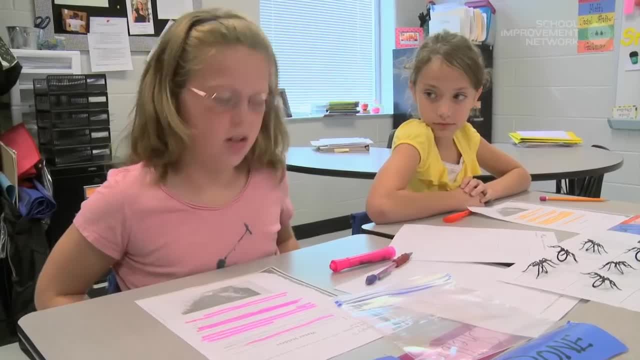 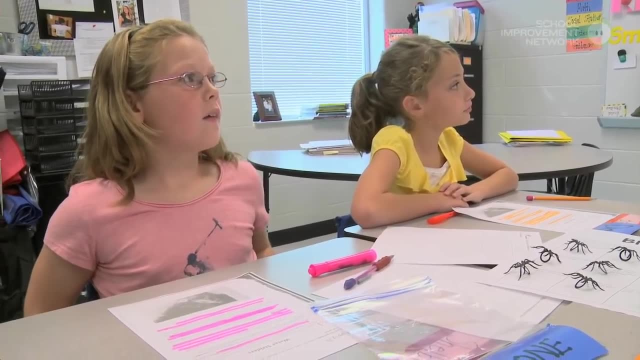 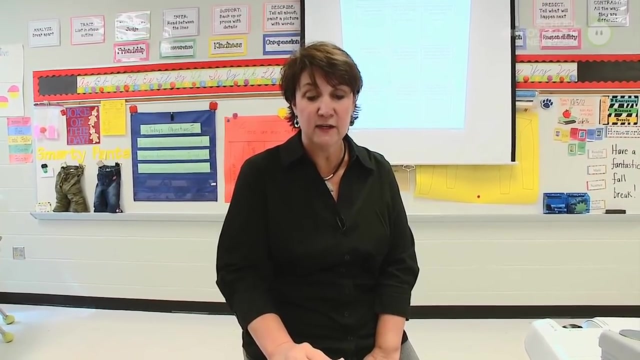 So how would you classify it? It is a what An insect. It is an insect We had to work on. classify, Okay, classify. And then the last one for the day on questioning is: what information would you use to support the view that water sharders spend most of their time on?